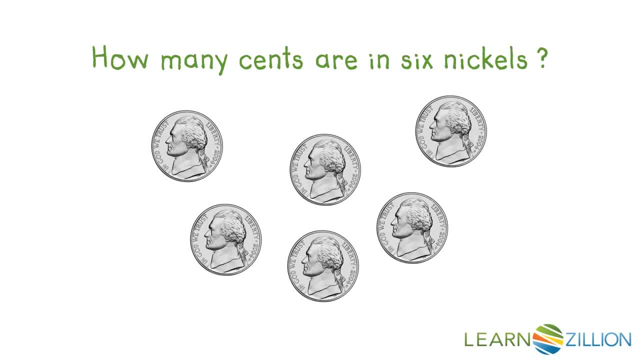 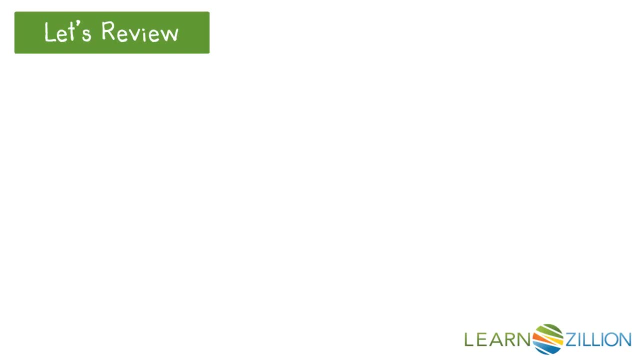 How many cents are in six nickels? In this lesson, you will learn how to count money by skip counting, Let's review money. Here we have a nickel. Remember, nickels are worth five cents. This coin is a dime. A dime is worth ten cents. This: 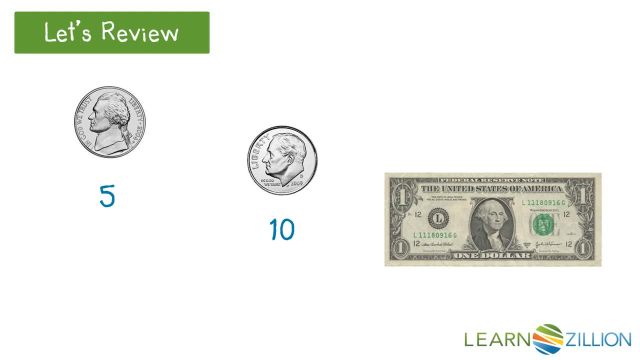 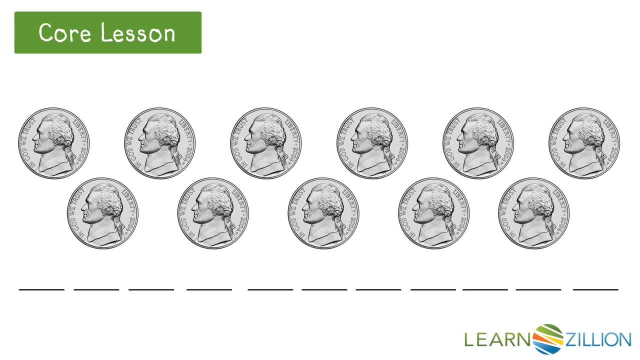 is a one dollar bill. One dollar is worth 100 cents. There are 11 nickels here. Remember each nickel is worth five cents, So you can count by fives to see how many cents all together: 5, 10,, 15,, 20,, 25,, 30,, 35,, 40,, 45,, 50.. Look at the 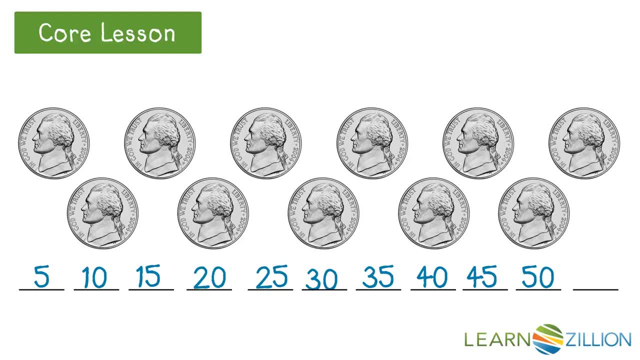 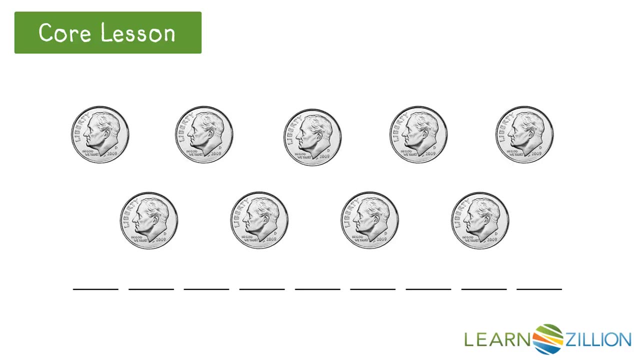 pattern. What number would come next? That's right, The number 55 is next. 11 nickels is worth 55 cents. There are 9 dimes. Remember each dime is worth 10 cents, So you can count by 10 to see how many cents all together: 10,, 20,, 30,, 40,, 50,. 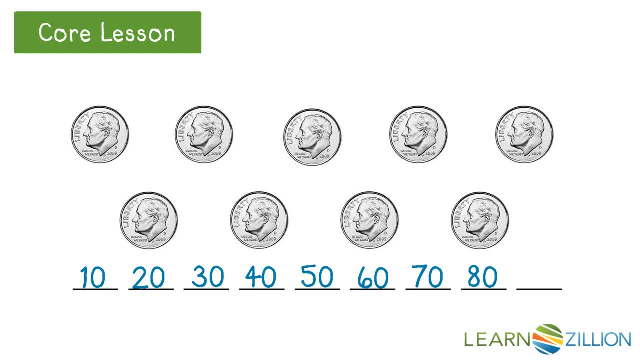 30, 40,, 50,, 40, 50.. Look at the pattern. What number would come next? That's right. We said there are nine nickels and there are five cents. Remember each dime is worth 60,, 70,, 80,, 90.. 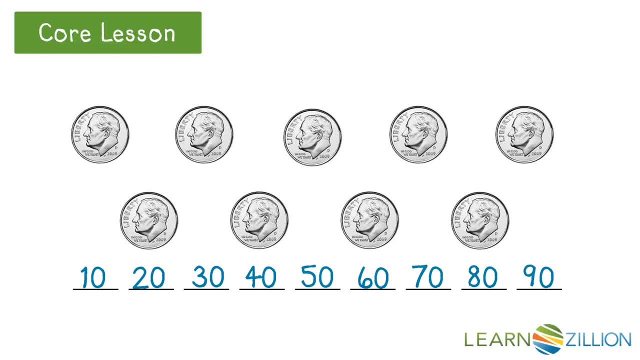 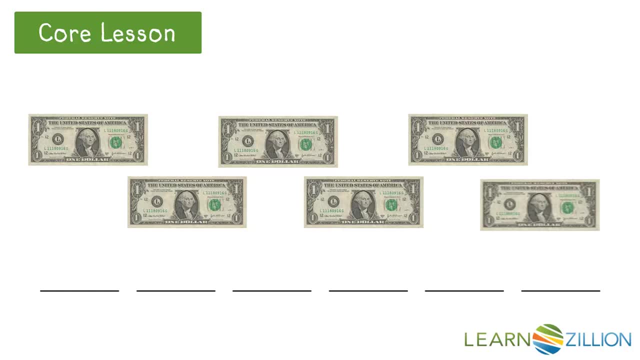 9 dimes is worth 90 cents. Here there are 6 $1 bills. How many cents is that? Let's skip count to find out. Remember, each $1 bill is worth 100 cents. So skip counting by hundreds will tell us how many cents there are. 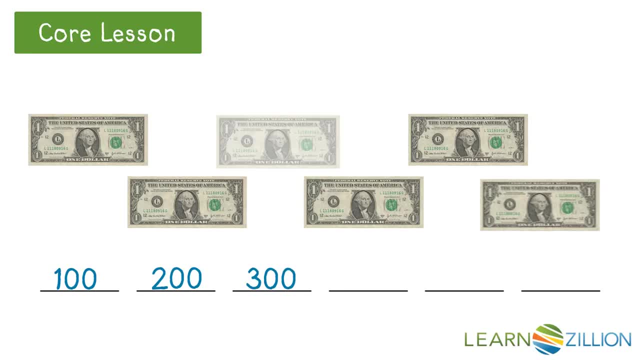 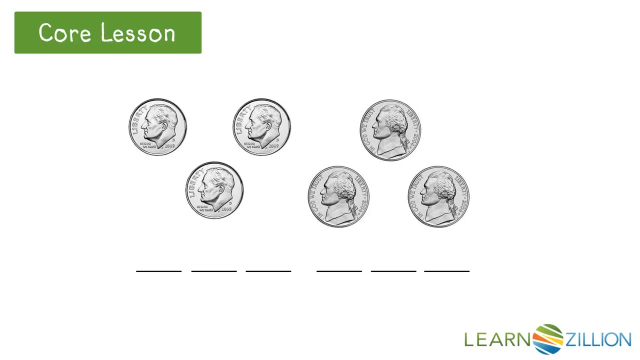 Here there are 100, 200, 300, 400, 500, 600.. 6 $1 bills is worth 600 cents. Erica has the following coins: She wants to know how much money she has. There are 3 dimes.